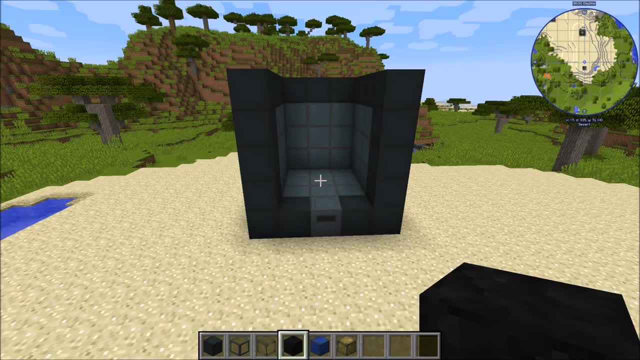 example. that's on the getting started guide on the official FTB wiki. So if you prefer a sort of text version of a tutorial, then head over to that page. It's a really nice page to get you started with nuclear craft. So this is. 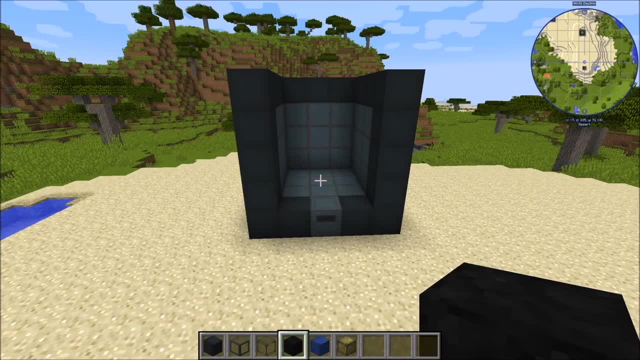 effectively just the video version of that. So what we're going to do is first of all, try and work out how many cells we can get away with putting in this reactor. So the first thing we want to think about is the fact that we've only 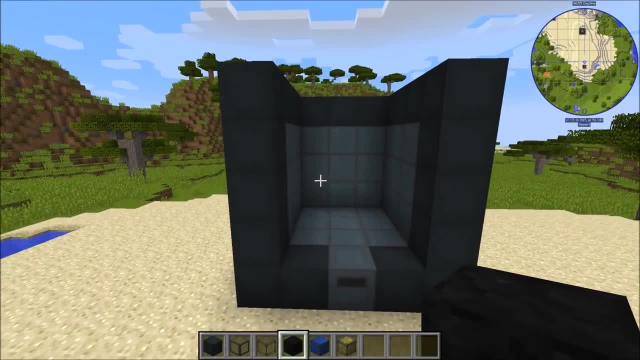 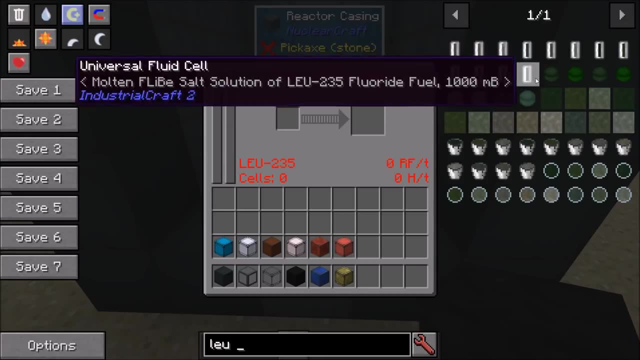 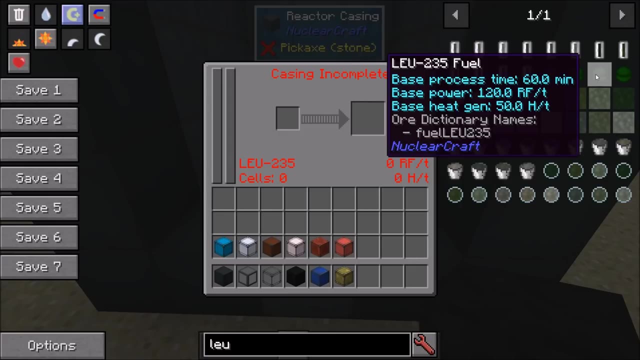 got 27 spaces inside of this reactor and we know that the base power of this LEU-235- if we check quickly, LEU-235 is 120 RF per tick but, more importantly, the base heat is 50 heat per tick. All right, now, 50 per tick is not that much really, because if we look at these, 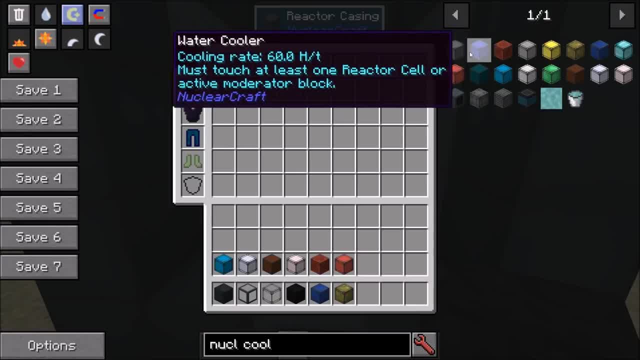 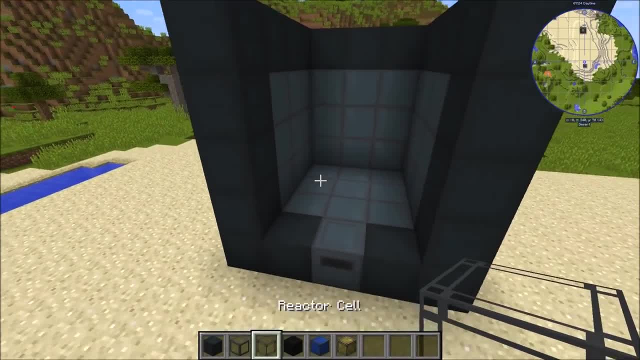 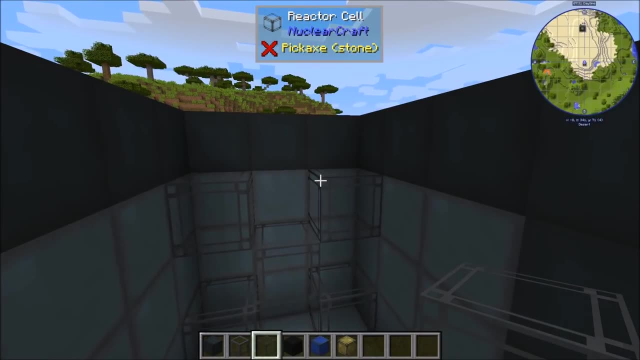 coolers, you'll see that most of these coolers usually can cool at around the 100 per tick roughly mark. Now let's imagine, for example, that we put, like, say, five cells in like this: not touching well, that would generate 250 heat per tick and we still have 22 spaces in the reactor. 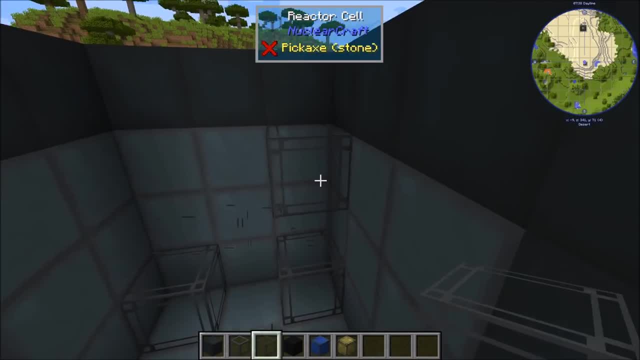 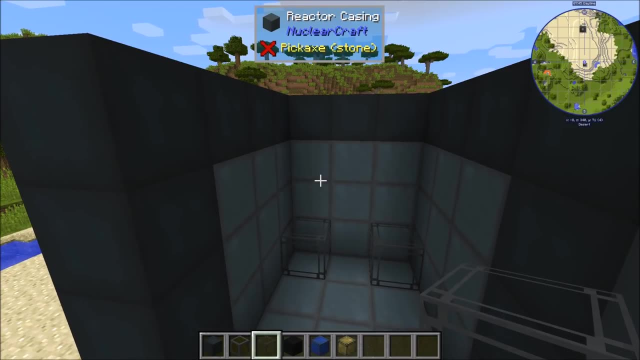 so that's definitely enough space to deal with that sort of amount of heat. so the first thing to do is sort of try and work out how many cells and graphite you can get away with putting in the reactor. now, if you do, the calculations just go through in your head quickly. let's imagine we 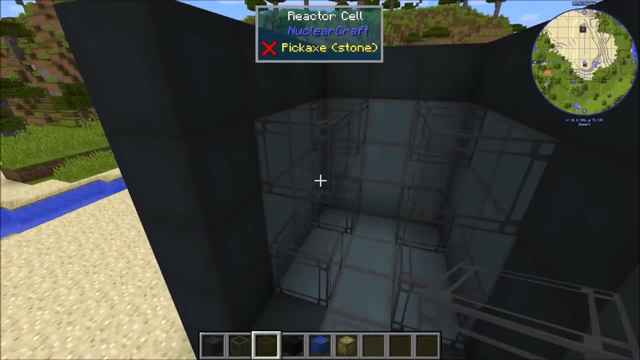 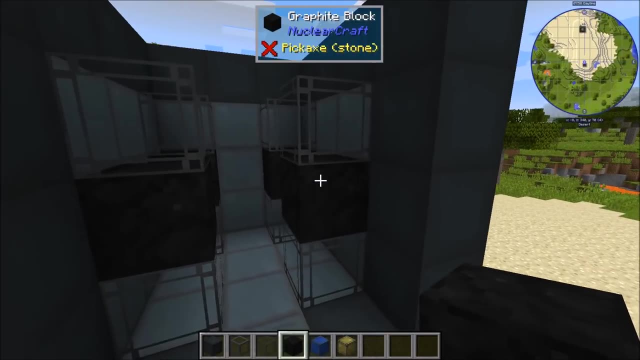 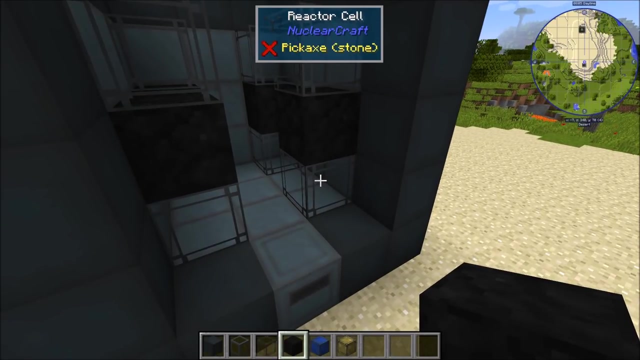 try to put four pillars of two cells connected with graphite, so each of these is basically going to be whatever amount of heat this pillar produces, multiplied by four. now each of these reactor cells are going to have an efficiency of two. that means they're going to be producing three. 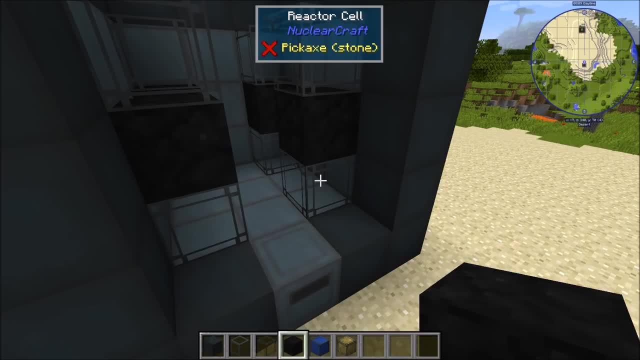 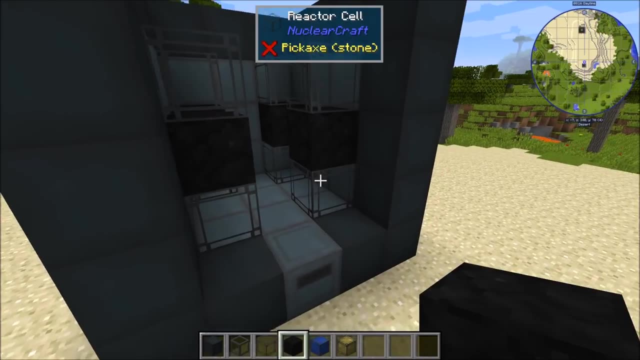 times the amount of heat, because, remember, the amount of heat that a cell generates goes up as the triangle number of the efficiency. so these are both going to producing three times the amount of heat, which is 150 heat per tick each. and then the graphite block, remember the. 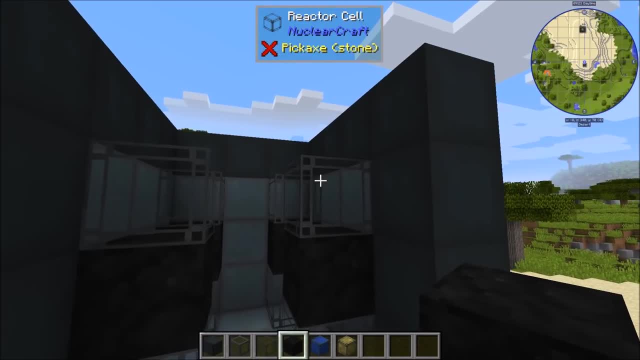 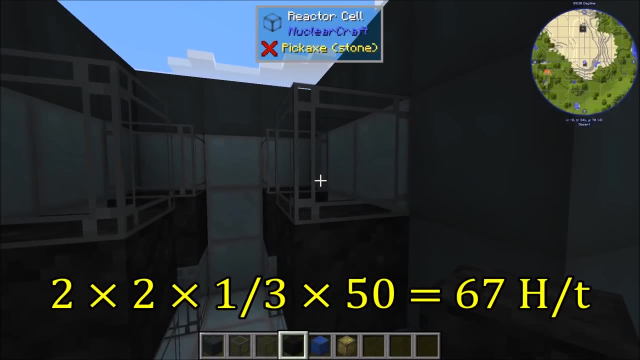 rule for that is that it's one third times the base heat of the fuel multiplied by the efficiency, so that's two thirds for each of the cells times the base heat, so that's four thirds times the base heat, which is around 60.. so in total, this pillar is going to be generating. 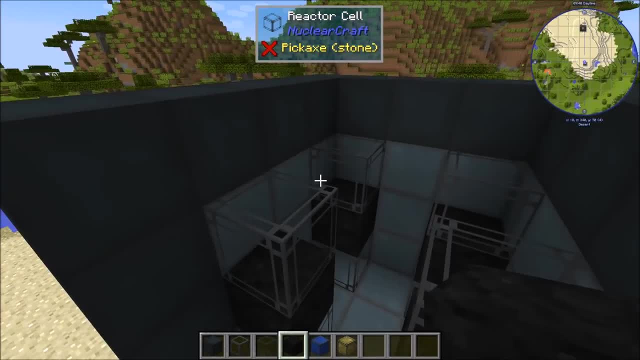 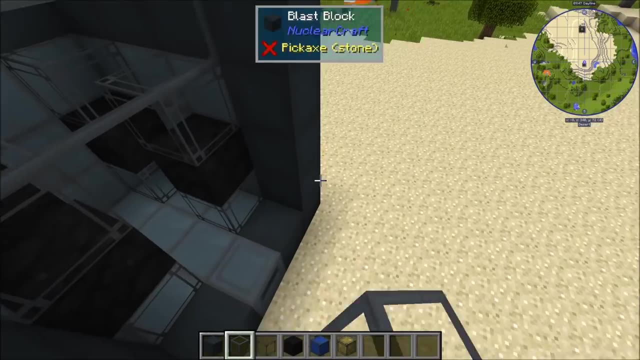 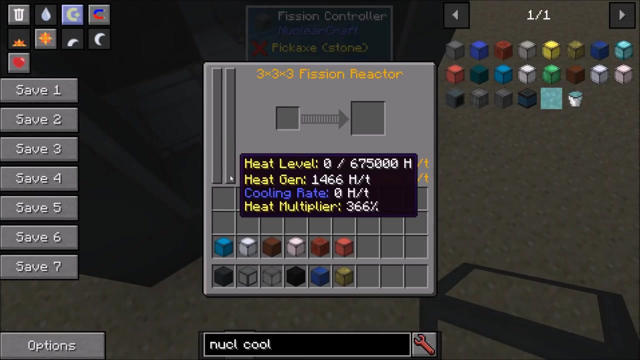 around 360 heat per tick. we can multiply that by four and we get 1440 heat per tick. now we can actually just test that quickly by putting some reactor casing to complete this structure. oops, and we can see here that we are generating. we check in the heat per tick: about 1400. 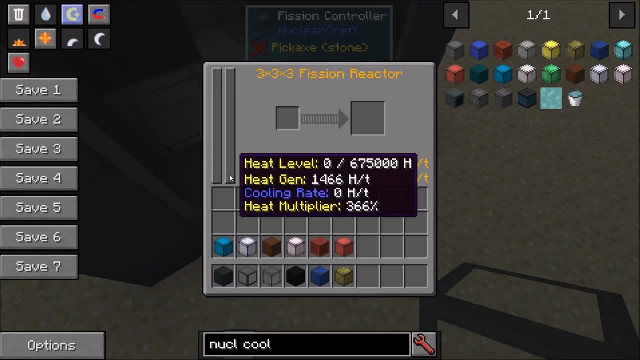 1440, 1466 heat per tick. so obviously you can just use the gui to actually check how much your design is going to generate. now we can use that number, the 1466 heat per tick, and determine whether or not we have enough space to to make the cooling viable. so we've used up 12 spaces in here, one, two. 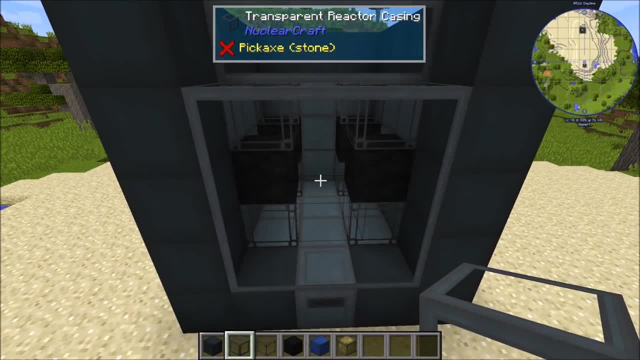 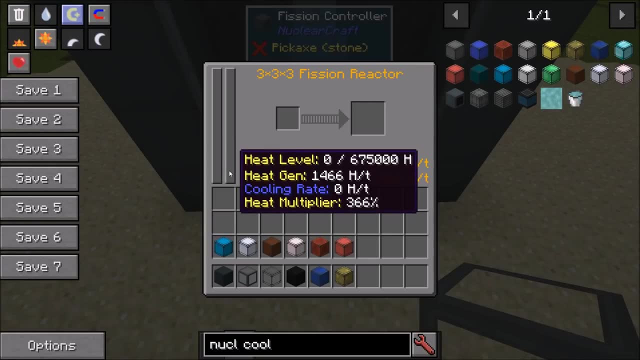 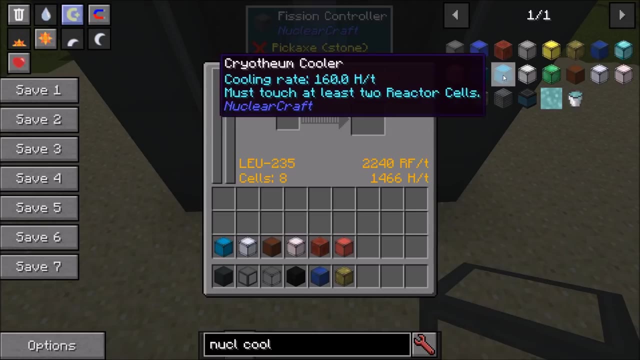 three, four, five, six, seven, eight, nine, ten, eleven, twelve, and we have a total of 27. that means we've got 15 spaces in there for coolers. now that means that we're going to need roughly 100 heat per tick. as you can see here, most of these reactors, most of these coolers do cool at around 100 heat per tick. 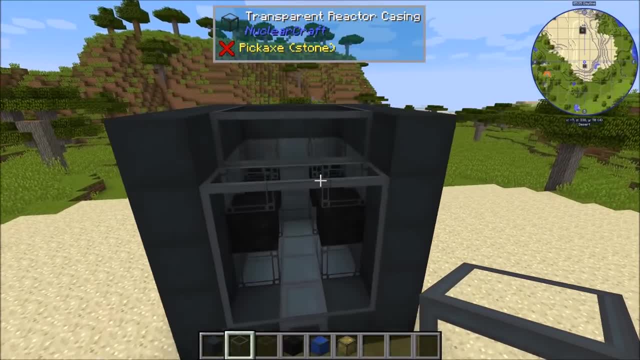 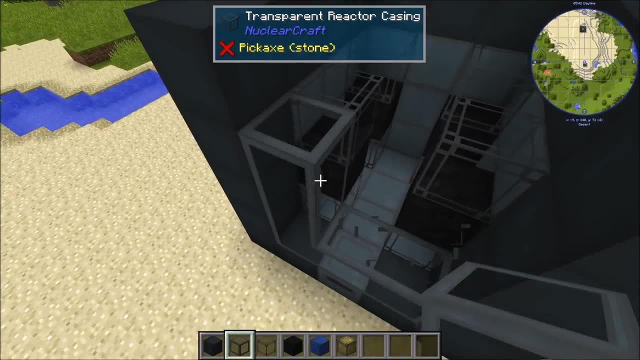 so i'm going to say that this is a design that might be worth trying out to cool, so let's get going with that. so the first thing to do would be to try and work out which coolers are best next to these cells. now there are a couple of options that we could go for. we could go for: 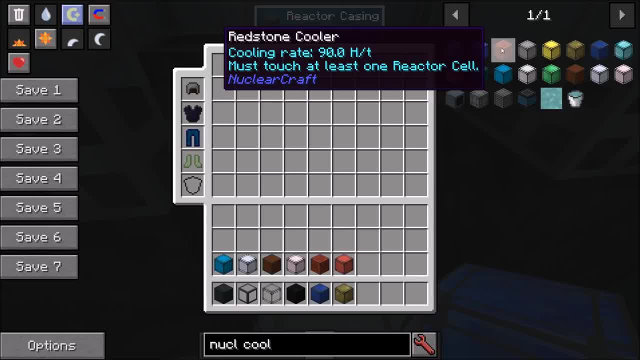 redstone coolers which must touch at least one reactor cell. we're going to start cheap. we're going to start with basically just these coolers here. i'll show you why, basically just for the purpose of the tutorial. but we're imagining this is sort of early game. you don't have access to a lot of cryo human stuff yet, so our option might be a. 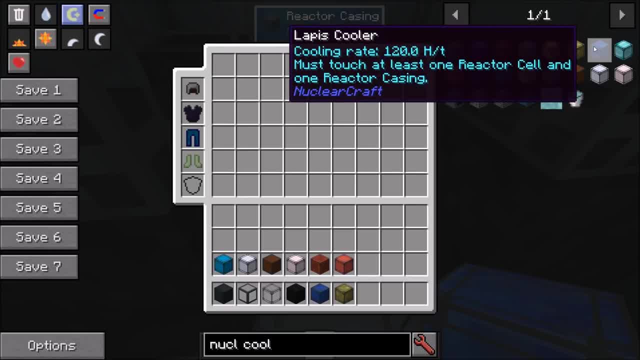 redstone cooler, but the better option is actually a lapis cooler, because that has to touch at least one reactor cell and one casing and all of these spots next to cells are viable for that, and it calls at a rate of 120 heat per tick rather than 90. so that is the better option, and so we will. 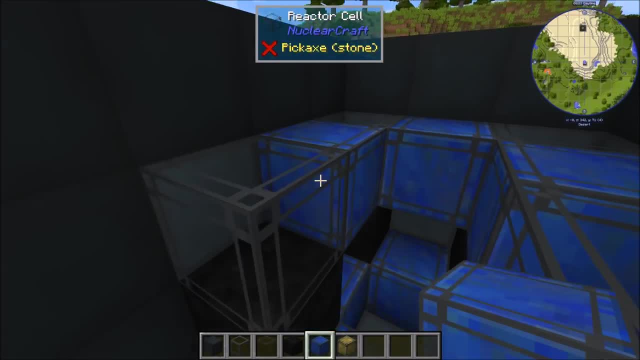 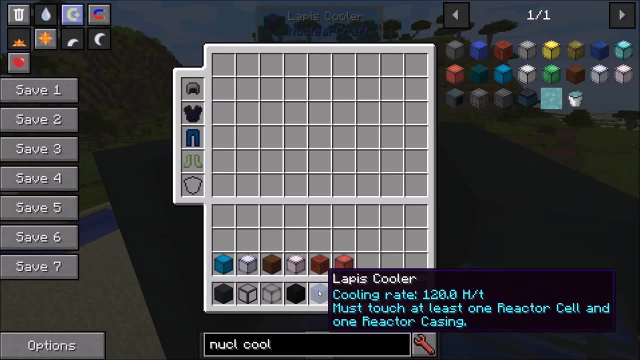 put eight lapis coolers down here, and so already that's eight times 120, which is nine hundred and 160 heat per tick. so already we've done quite a lot of the cooling that we need to do. we only need to do about 500 heat per tick more cooling. the next thing to look at is the spaces between: 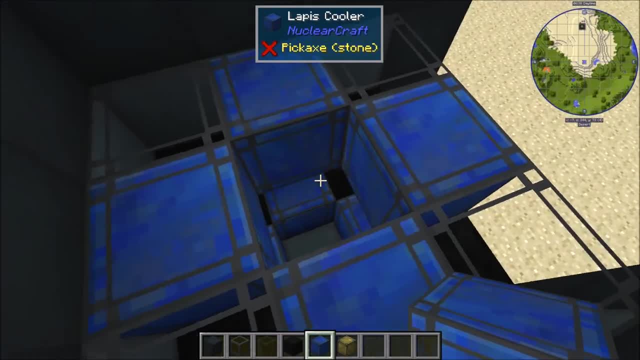 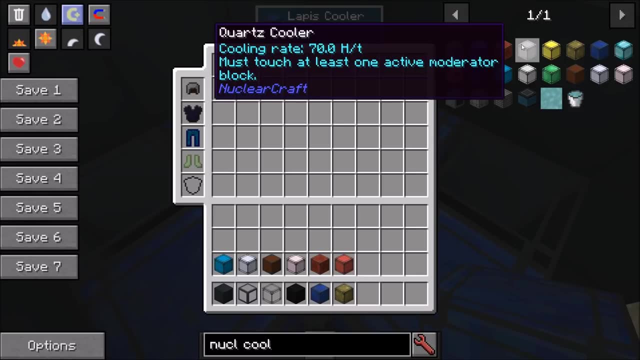 these graphite blocks. now there's an obvious candidate for this. since there are two graphite blocks adjacent to each of these spots, we could go for a quartz cooler. that's 70 heat per tick must touch at least one active moderator block, such as graphite, but the glowstone cooler is: 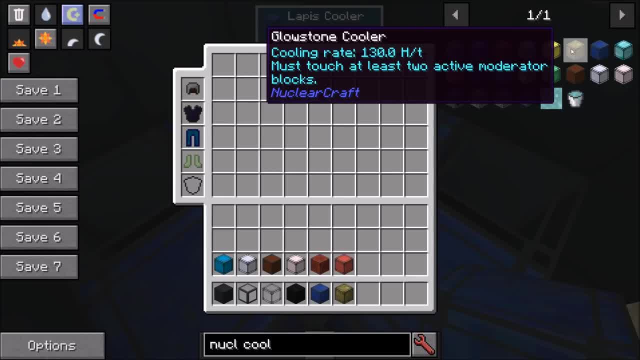 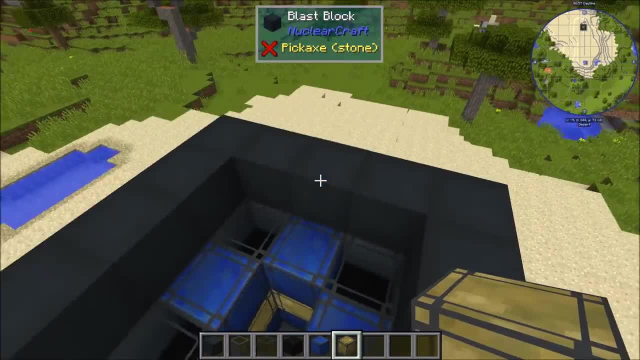 obviously the best thing to go for 130 heat per tick and must touch at least two active moderator blocks. so this is clearly the best thing to go for in this particular case. so we can put these in there now. if we check the amount of heat that we're generating in our reactor, we will find 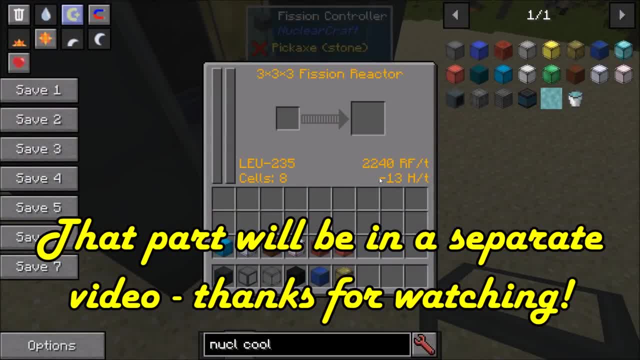 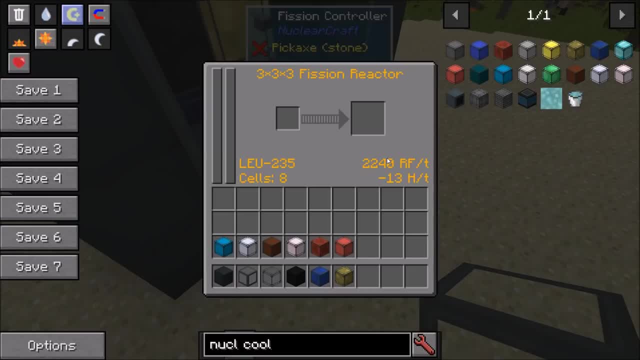 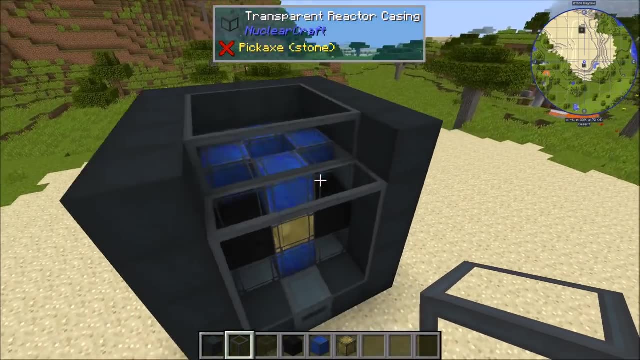 that we're doing all the cooling that we need to do, minus 13 heat per tick overall, which means that our reactor is net negative on heat and we're producing 2240 rf per tick. so this is a totally stable lu235 3x3x3 reactor. so that's brilliant. we really do not need to do any more cooling. 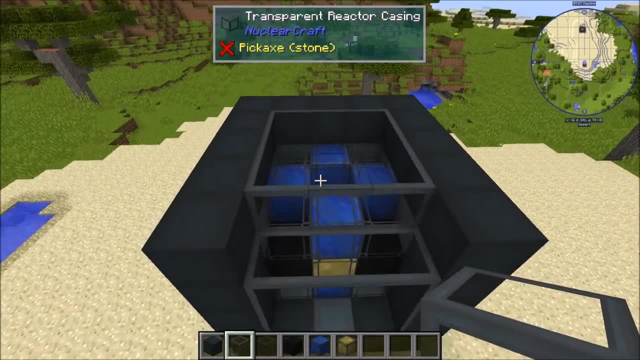 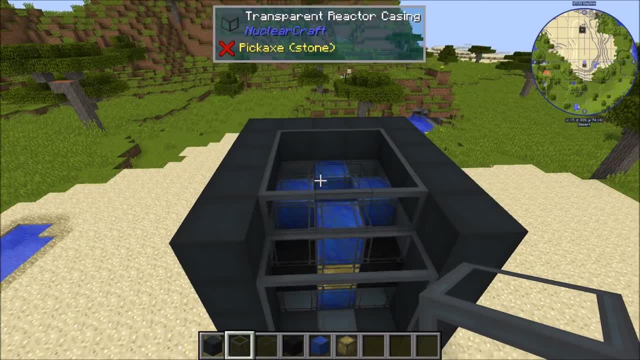 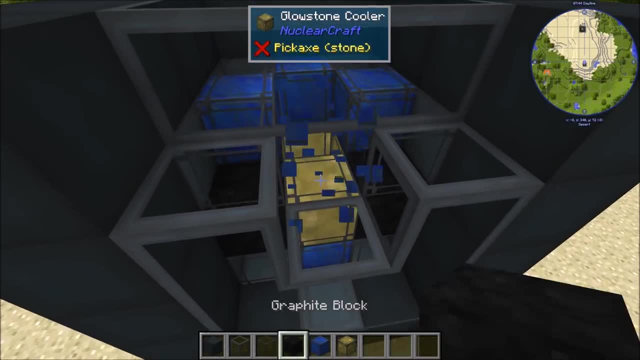 expensive coolers, cryo fium, liquid helium, etc. etc. let's try and imagine that we wants to just beef up the amount of power that we producing and we did something like putting an extra graphite block here instead of a lapis. now, when we close it back up again, we'll see the amount of power that we're. 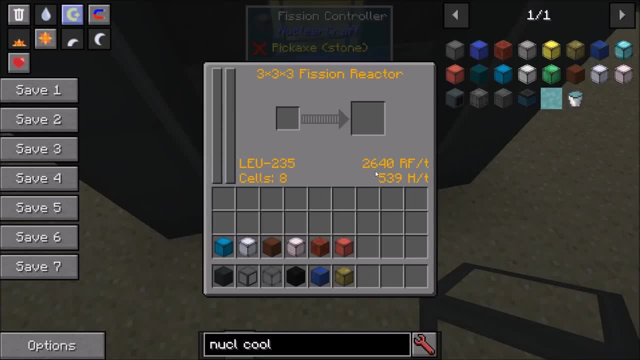 generating is a bit higher: 2640- so that's about a 20% increase in the power. so that's that's. that's pretty good. but we can see here that we've got another 540 heat to deal with here. so that means that as it stands, our design is certainly not going to be good enough, because we've only got 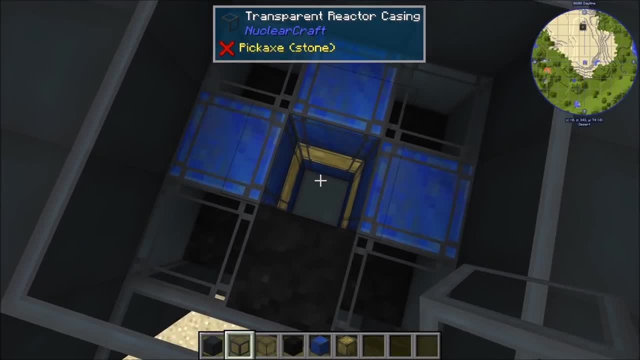 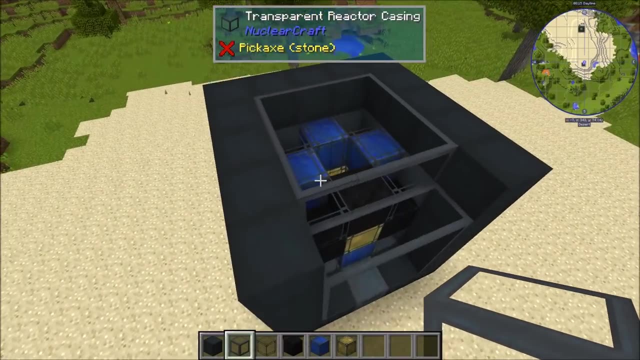 three spaces life left, and that means that we're going to need about 180 heat per tick of cooling, and none of the coolers reach that sort of level. so we're gonna have to go back through the design and check where we can improve things. so the obvious place to start would be those lapis. 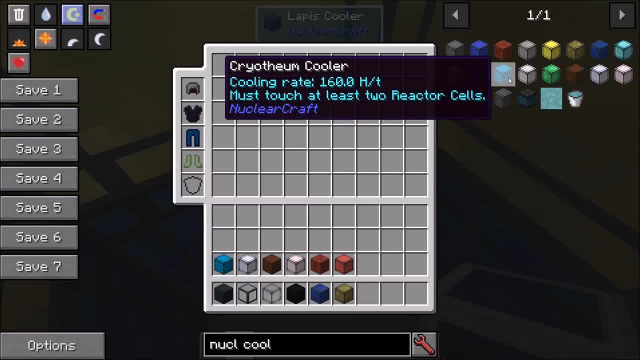 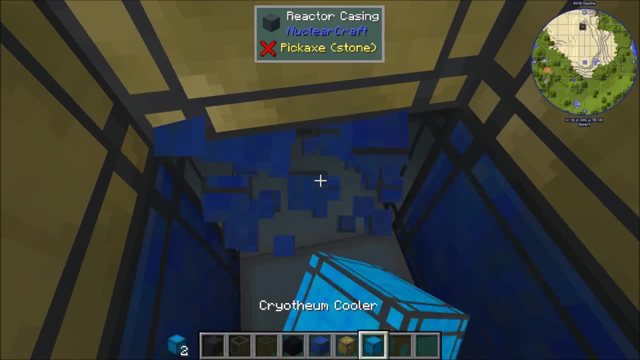 coolers on the bottom here. we can see here that the cryo fium cooler is a lot better- 160 heat per tick and must touch at least two reactor cells. so first of all we'll replace two of these lapis coolers with the cryo fium. now why do I only replace two? well, because we can also look. 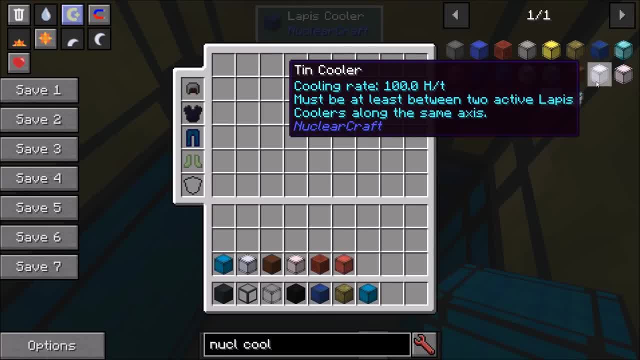 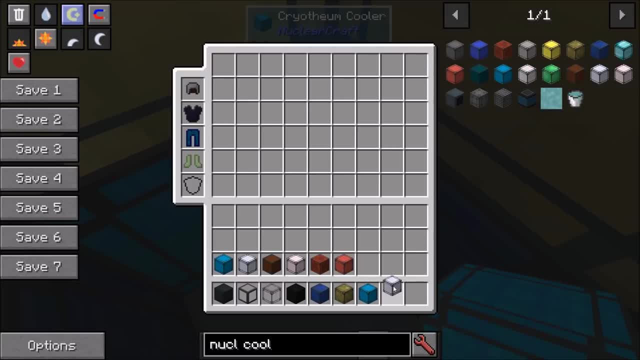 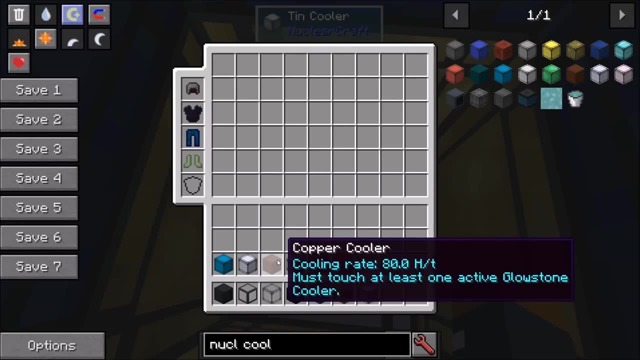 over here at the tin cooler, which must be at least between two active lapis coolers along the same axis. so I've got two lapis coolers along the same axis here, and so this means that a tin cooler can go here. there we are. next thing to look at is the copper cooler. the copper cooler must touch at 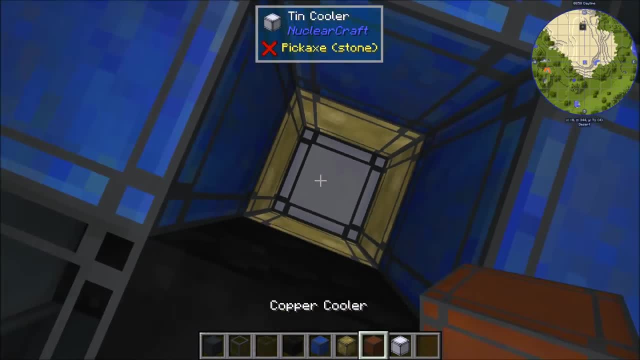 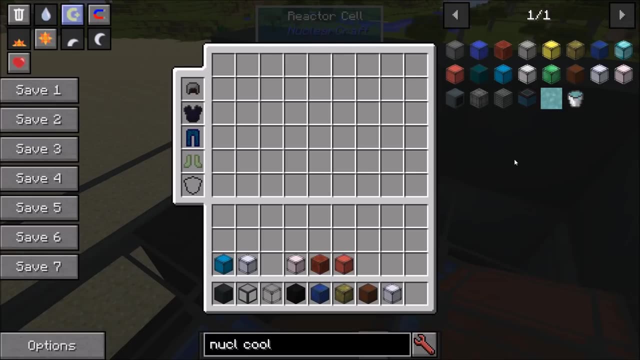 least one active glowstone cooler, and so that is the obvious option here. next to all those glowstone coolers, and then finally, on the top, we have this extra graphite block to work with, and so perhaps we want to go with a magnesium cooler, which must touch at least one reactor casing while it's on. 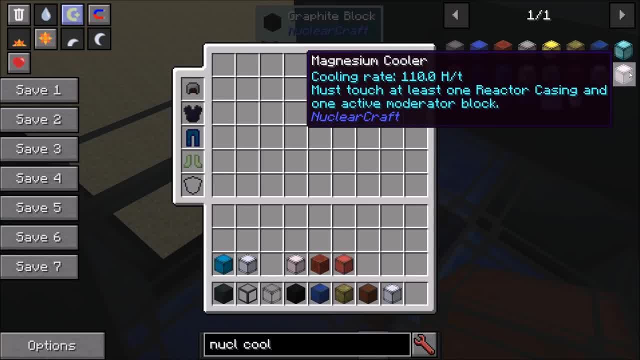 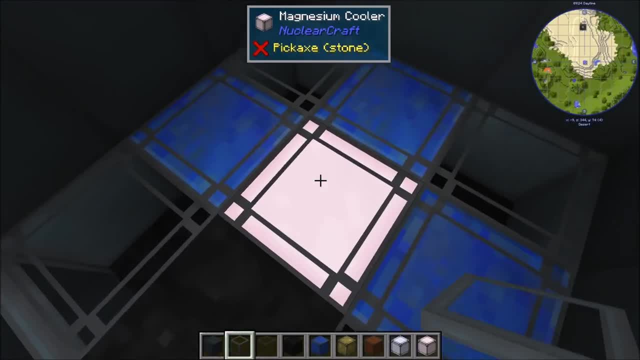 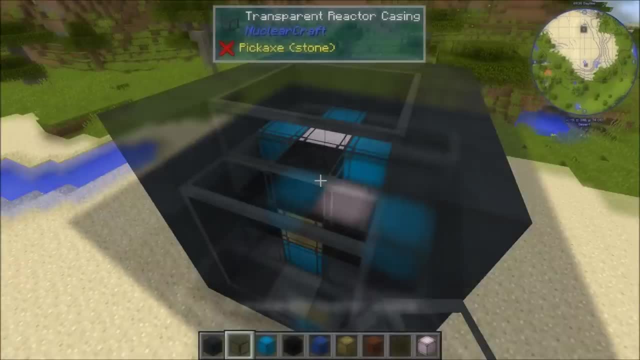 the top of the design, so it will touch a casing and needs to touch an active moderator block as well. so again, that's absolutely fine. of course, actually, what we could also do is replace these lapis coolers with cryo fium as well. so let's do that quickly, let's see. 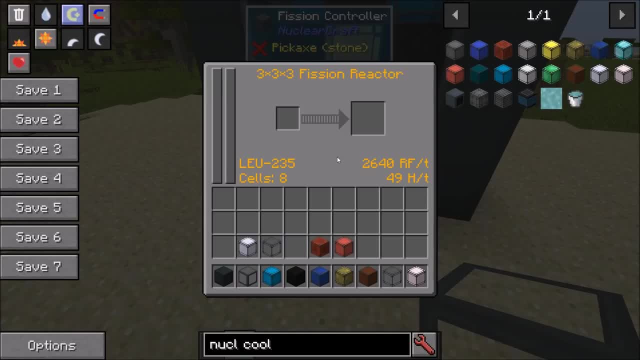 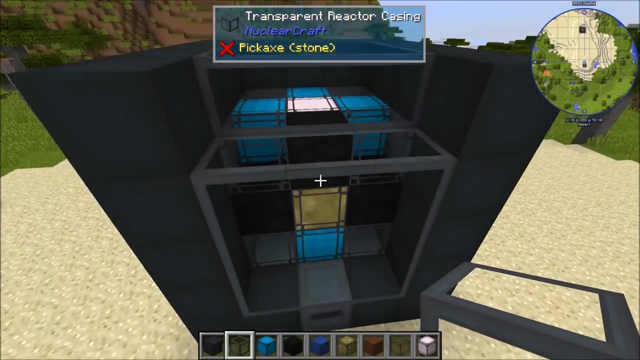 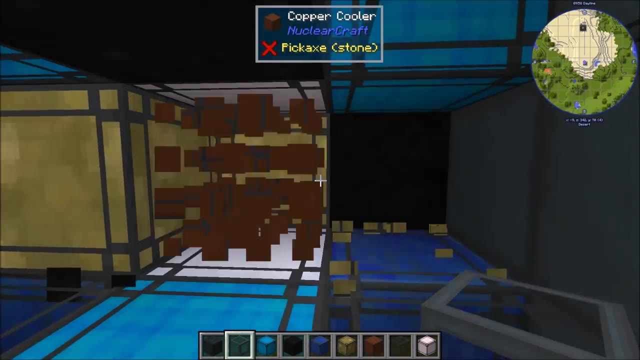 still not quite enough: 49 heat per tick left. so we're going to still have to go back inside and work out if we can improve things. I'm wondering, on the bottom there we could deal with those lapis coolers. so if we go back underneath here and just dig away, just destroy this and we'll put it back, 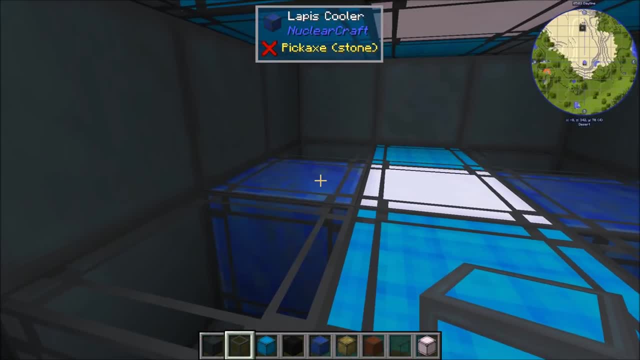 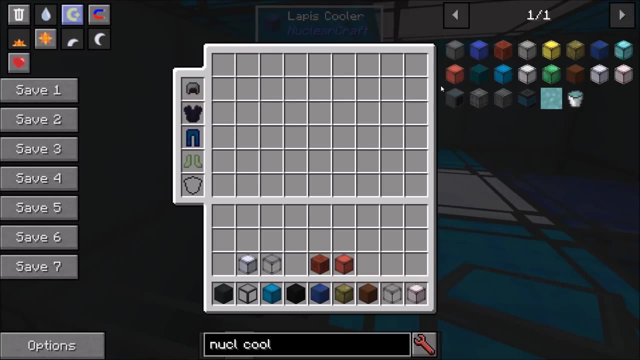 but if we look here perhaps we can actually improve on this. so let's go back through the coolers that we have available. we have the redstone that we didn't think about before. the redstone can actually support a liquid helium cooler, so that needs to touch at least a reactor casing, so that's a possibility in the middle here. 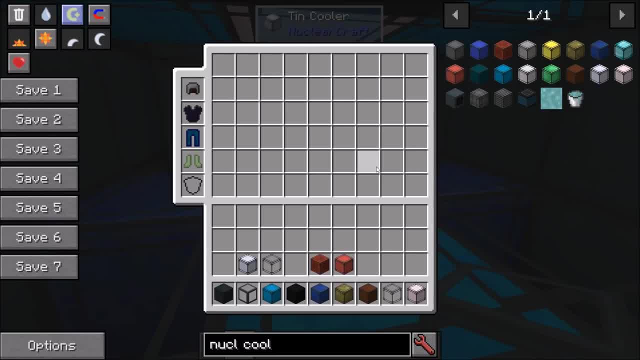 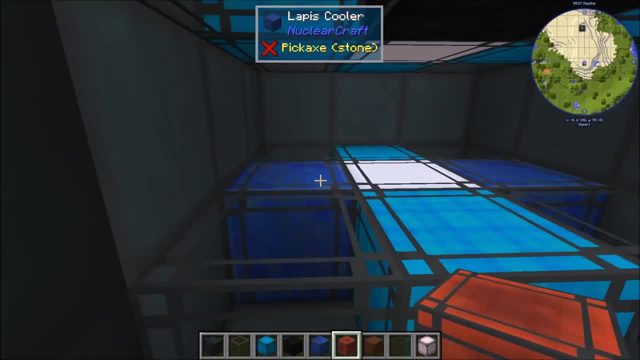 and it needs to touch a redstone cooler, so maybe we should get a redstone cooler in. so first of all, we're gonna have to replace a redstone cooler. well, we're going to. that means we're probably gonna have to replace one of these lapis coolers, so we might as well replace both of. 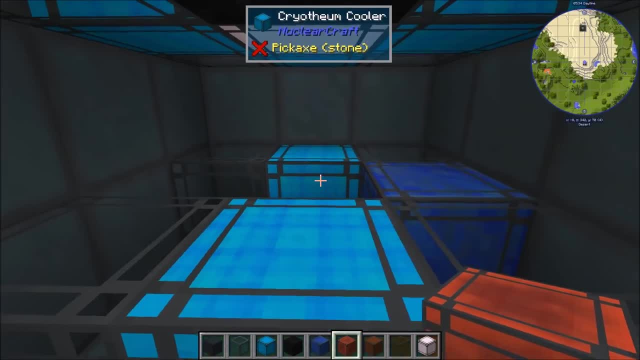 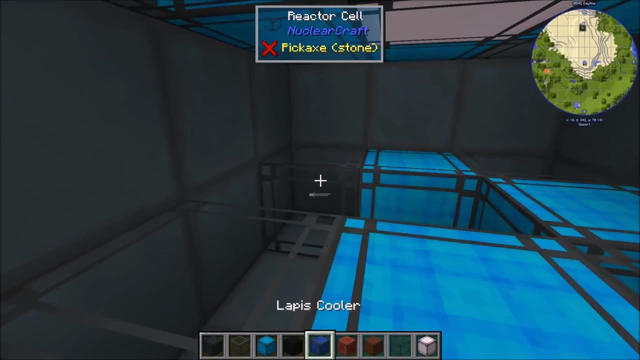 them, because this tin cooler is not doing anything and it has to go anyway for the space for the liquid helium and we can now replace this other lapis cooler with a cryo fium. so that's an improvement of 40. already. that's a good start. so before we had a tin and lapis, that's a total of 100 plus 120, so it's 220. 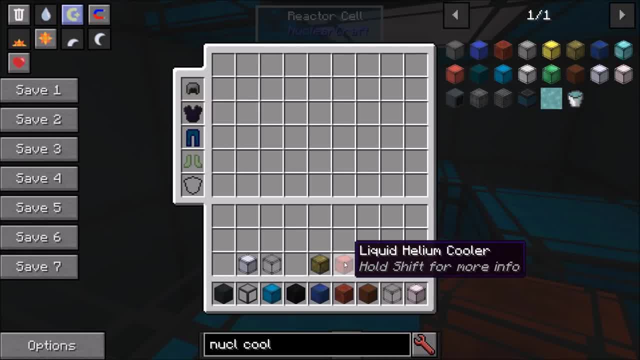 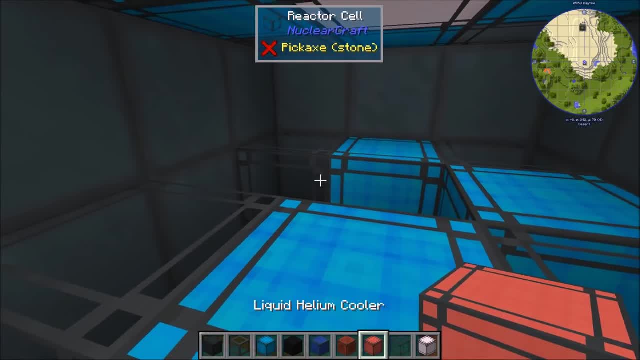 heat per tick and we're going to be replacing it with 140 plus 90, which is 230, so that's an extra 10 plus an extra 40 from the cryo fium. that must mean that surely we should just be able to cool.